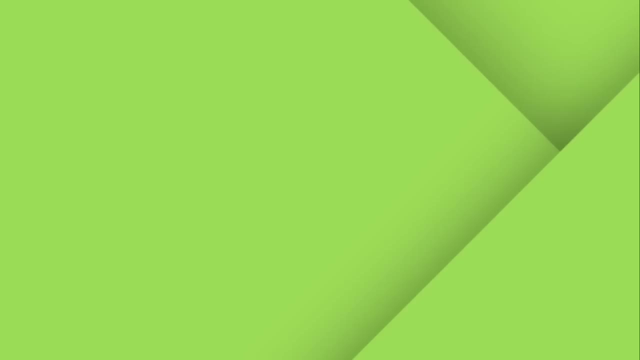 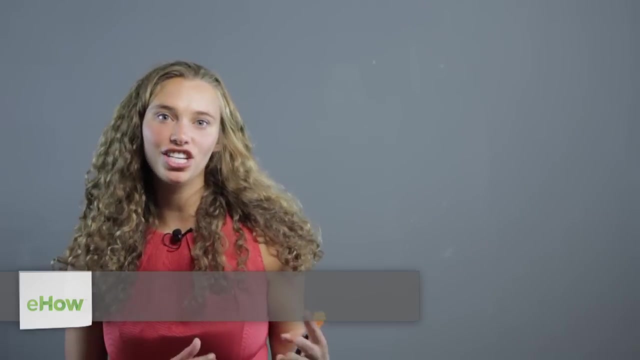 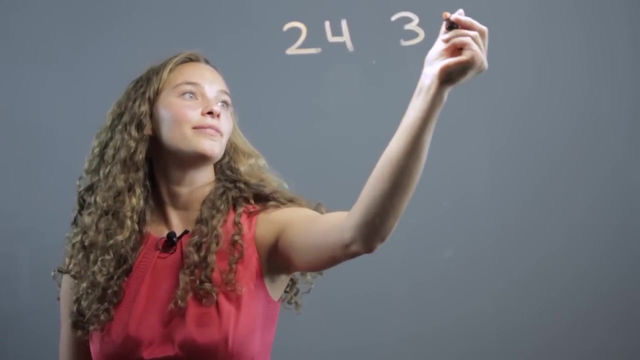 Hi, I'm Rachel Kaplow, and today we're going to be going over how to teach LCM and GCF using the Ladder Method. Let's look at the numbers 24 and 36.. So now we want to find the LCM and the GCF. 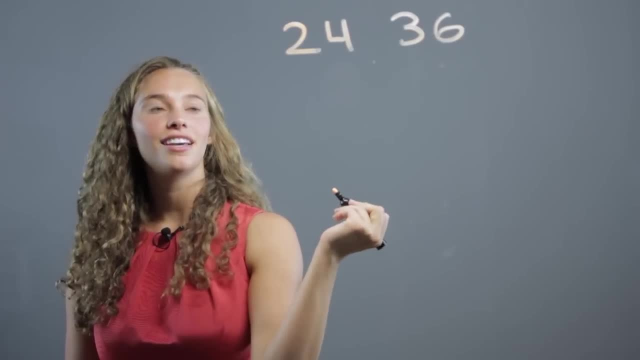 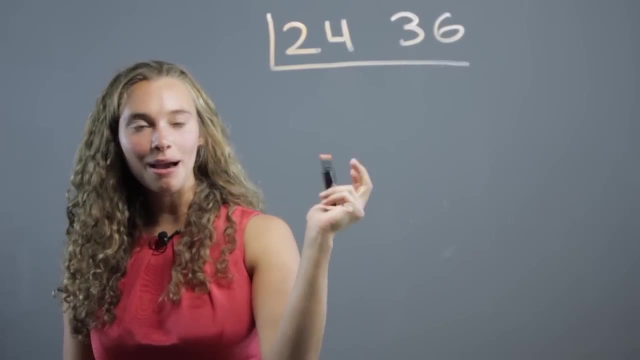 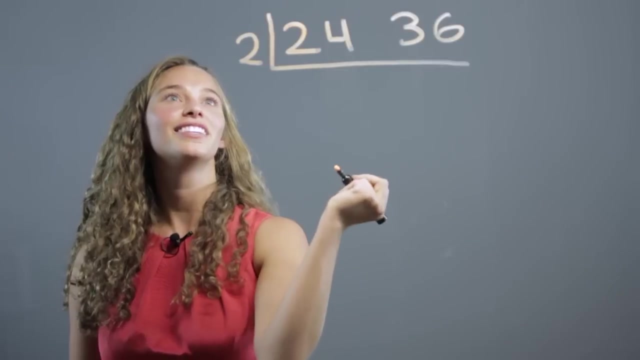 Start off by writing the numbers on one line like this. Then make an L Ladder Method. Now we're going to find the smallest prime number that goes into these two numbers. In this case it's 2, the smallest prime number. 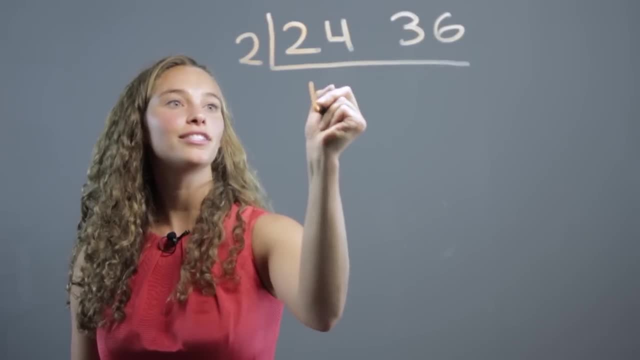 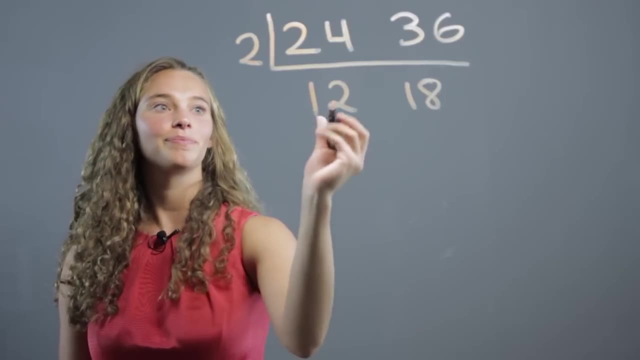 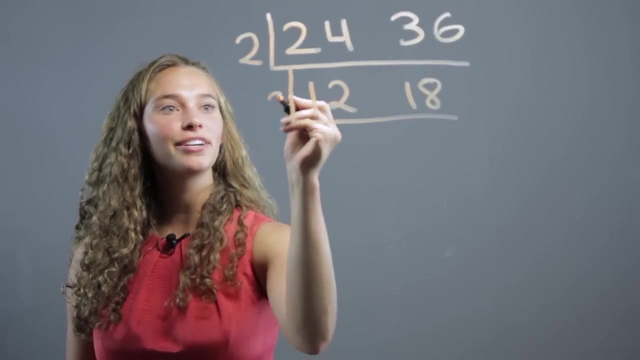 So we have 2 into 24 is 12, and we have 2 into 36 is 18.. Then we do it again until we have all prime numbers. So we make another L Again. the smallest prime number is 2.. 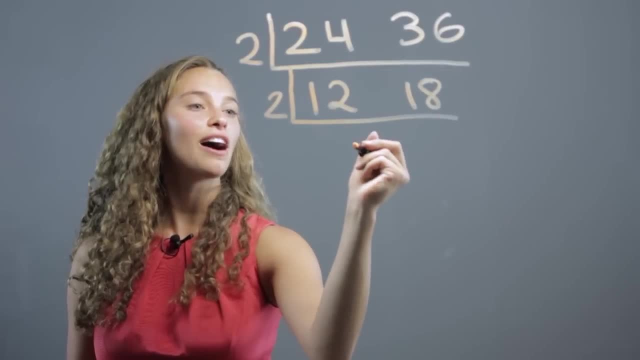 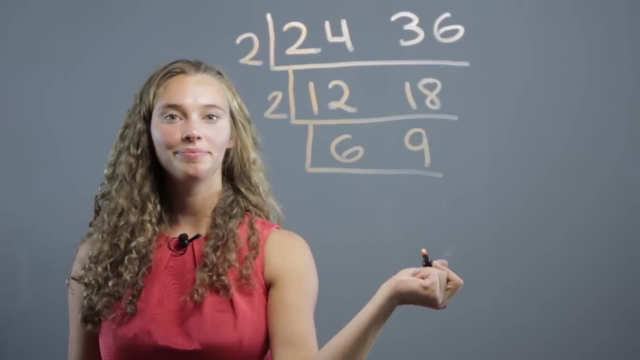 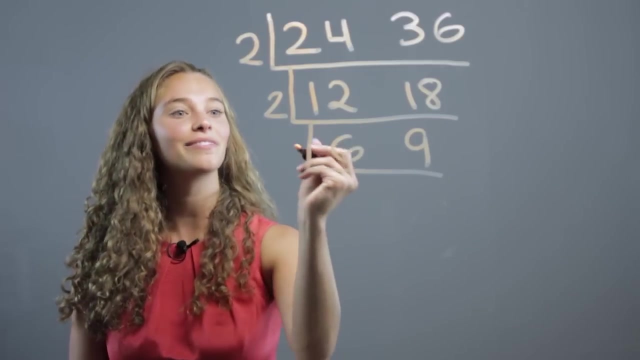 So we divide 2 into 12 to get 6.. We divide 2 into 18 to get 9.. Again, we make the L Now the smallest prime number that goes into 6 and 9, it's not going to be 2,, it's going to be the next one, 3.. 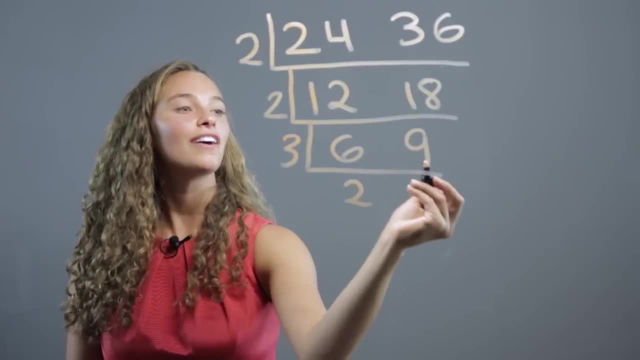 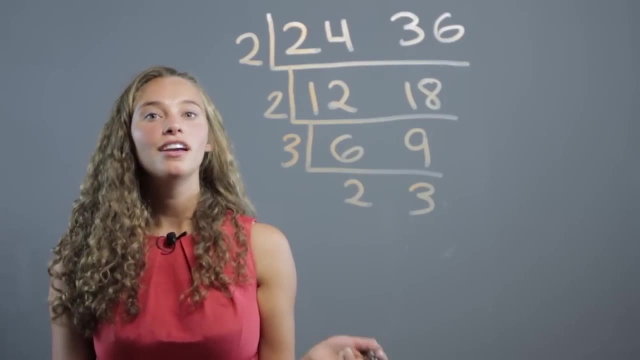 Divide 6 by 3 to get 2.. Divide 9 by 3 to get 3.. Now we have all prime numbers. so we know that we've finished. We're at the end To find the LCM, we make an L. 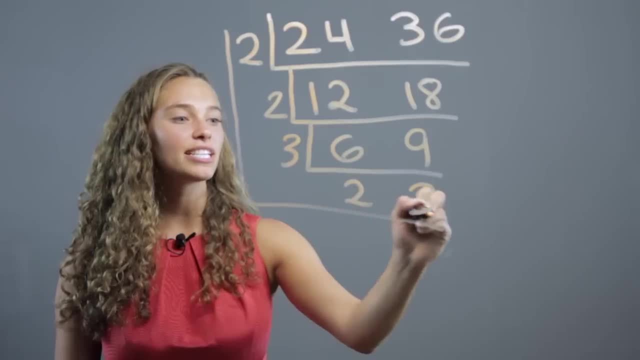 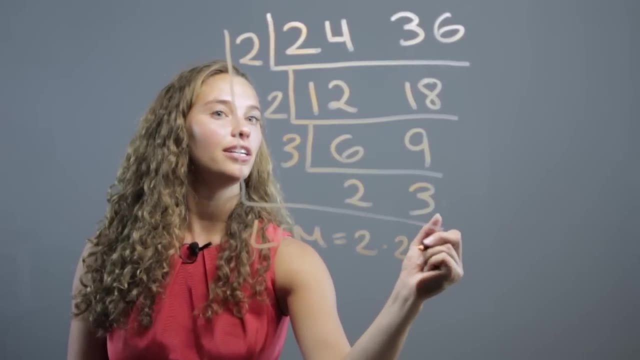 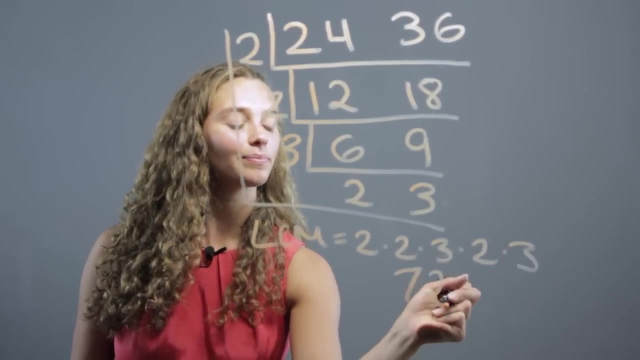 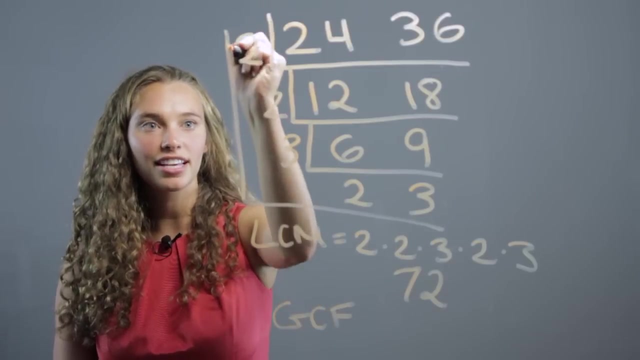 And we add, we multiply all those numbers together on the L. So LCM is going to be 2 times 2 times 3 times 2 times 3, which all together is 72.. The GCF we find by going straight down this line: 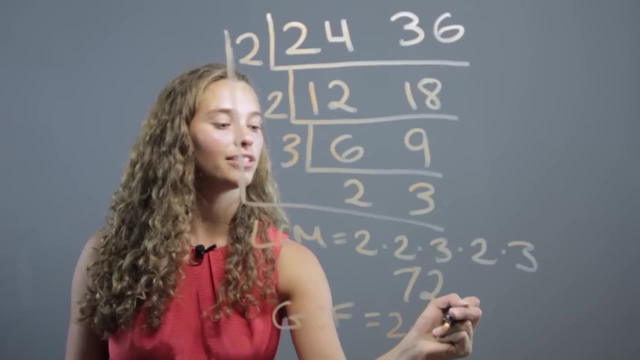 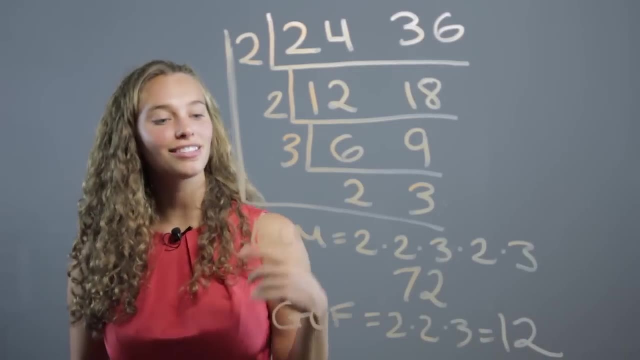 That's going to be 2 times 2 times 3.. 4 times 3 is 12.. And that is how you find LCM and GCF using the Ladder Method. I'm Rachel, and thanks for learning with us today.